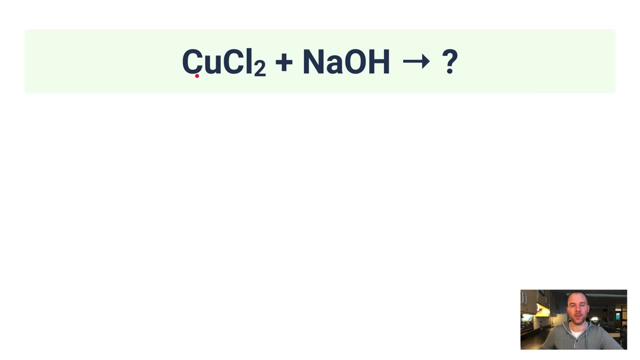 their products, and then we're going to look at some examples of double replacement reactions And we'll balance the equations. So this is copper 2 chloride- CuCl2, with sodium hydroxide, NaOH. Now it's a good idea to- and this is my suggestion- it's a good idea to, just above these, write the: 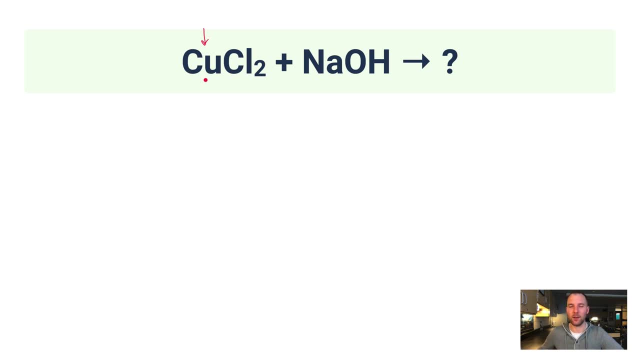 charge of each of these ions. So if you look at copper on the periodic table, it could be either plus 1 or plus 2, so you really have to look at what it's bonded with. Chloride is in group 17,. 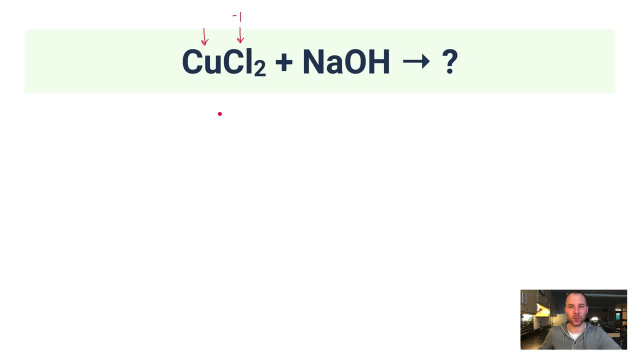 and therefore chloride will always have a minus. So if you look at copper on the periodic table, it has a minus 1 charge. There are two of them to balance out, whatever the charge on this one copper ion is, and so therefore that must mean that this 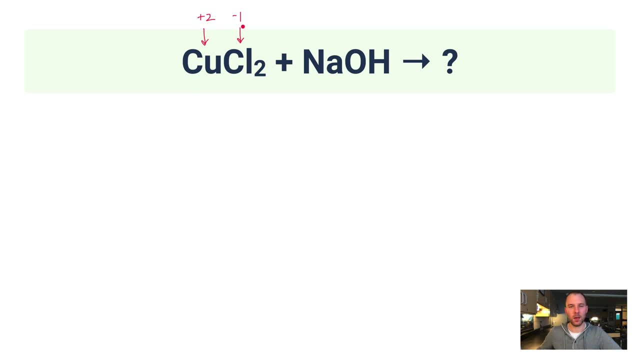 is copper plus 2, because 2 and 2 negative ones would neutralize this compound. So this is copper 2 chloride. Over here we've got sodium and sodium's in group 1. It's not a transition metal that's multivalent, so sodium is a plus 1 ion. 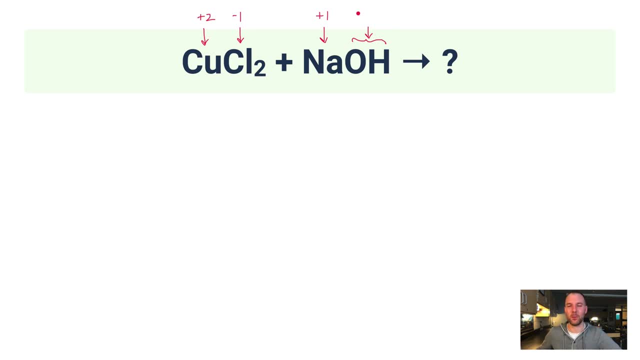 Here is a polyatomic ion. Table 5 will help you, or just a listing of polyatomic ions. if you're not taking my class and you don't know what table 5 is, This is a negative 1 ion. You can look that up. 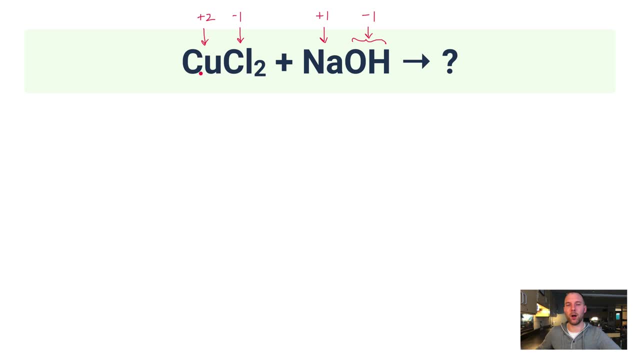 or maybe you'll have that memorized at this point. Now, this is going to help us figure out what the new product formulas will be, because what we're essentially doing is taking the front of the first formula and putting it with the back end of the second formula. 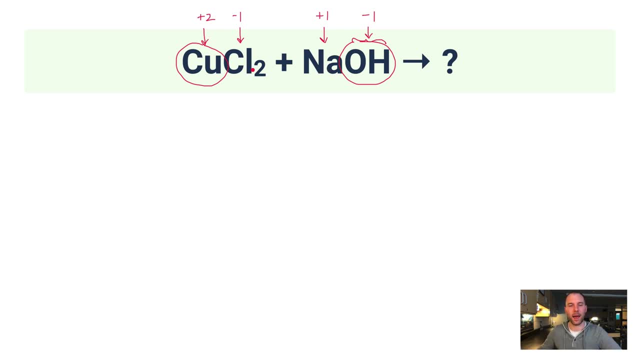 The same is true in the other direction. The front of the second formula will go with the back of the first formula. So let's put Cu2 plus and OH1 minus together first. Let's start by writing out our whole equation, because we're going to end up having to balance this too. So here are our two. 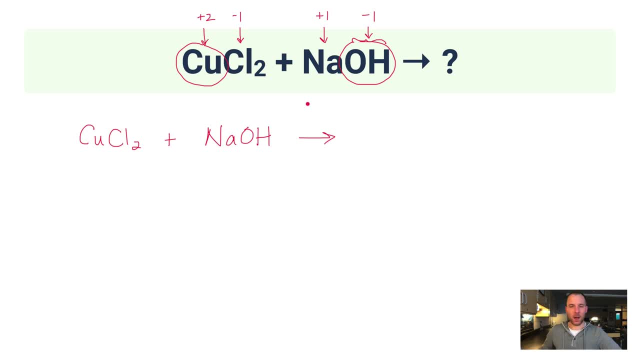 reactants. again, It doesn't matter what order you put the products or the reactants in. as long as they're on the right side of the equation, that's okay. Copper 2 plus with OH1 minus would form CuOH2,. 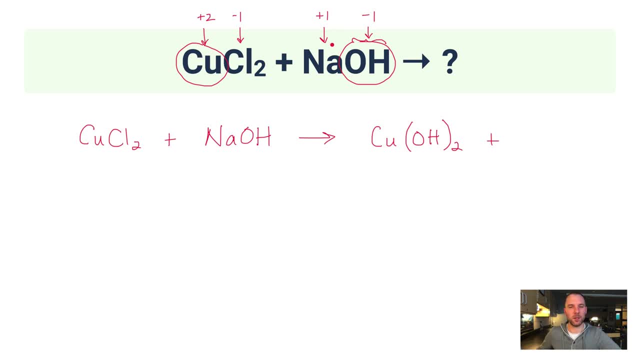 and then my other product is going to be sodium, Na plus 1, with Cl chloride, Cl minus 1.. So that's just regular NaCl. Okay, now, obviously you can see that this isn't balanced, so we have to balance this. Now I'm going to drop the line and list out all the elements on this one, but really at this. 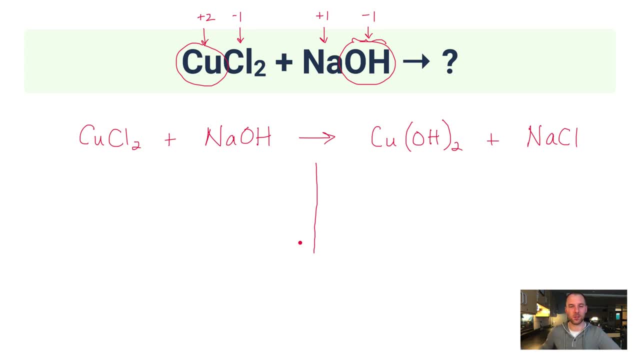 point. you should be faster at doing these. You might be able to just do this quick in your head If you need to skip ahead in the video to the next problem. But my suggestion with polyatomic ions, if they stay together like 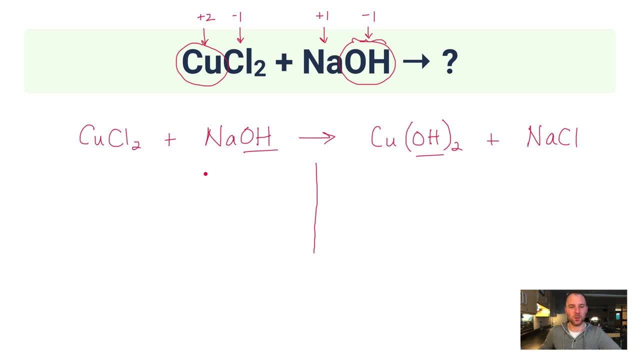 hydroxide does here is that you list it as if it's an element. So when I list out my substances in this, I'm going to list OH as though it's an element. It's a little trick: CuCl, Na and OH. Okay, on the left I have one chlorine or one copper, two chlorines. 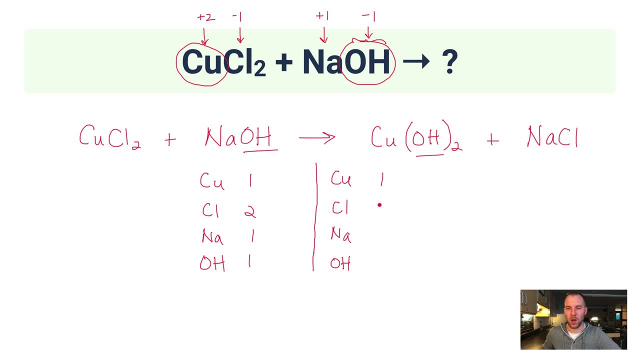 one sodium, one hydroxide. On the right I've got one copper, one chlorine, one sodium and two hydroxides, So you can start with the chlorines or the hydroxides, It doesn't much matter. On the right side, if you put a 2 in front of NaCl, that'll make each of these a 2.. 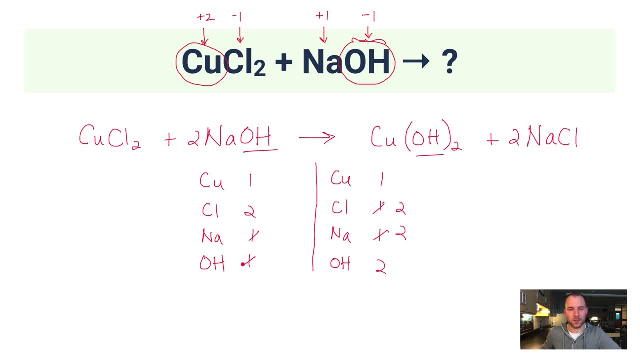 And then if you put a 2 in front of NaOH, that'll make each of these a 2. And that should balance the equation there. So that's it: CuCl2 plus 2 NaOH makes CuOH2 and 2 NaCl. 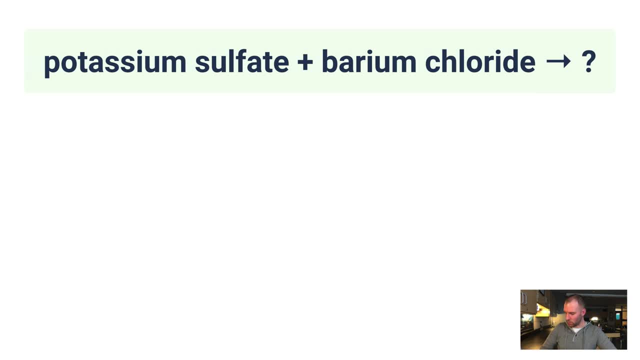 All right, here's another one: Potassium, sulfate and barium chloride. These are the names, so we have to come up with the formulas. So potassium is K, with a plus 1 charge because it's in group 1.. Sulfate again, if you need to reference that polyatomic ion list. 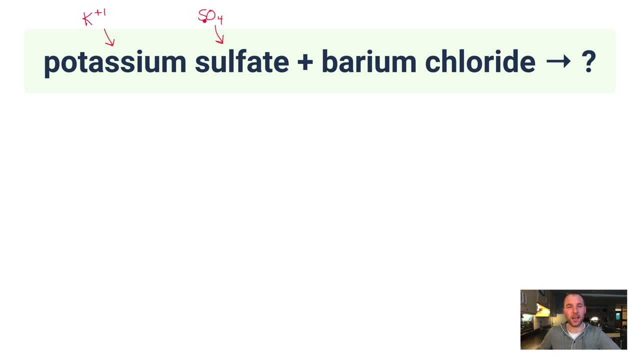 go ahead and do that, But you might have this memorized. Hopefully you do. It's SO4 with a negative 2 charge. Barium is Ba- It's in group 2, so it gets a plus 2 charge And chloride is Cl. 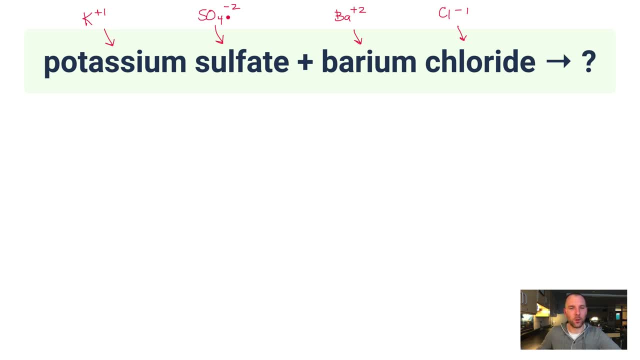 with a minus 1, just like in the last problem. So let's put together the formulas. Here are our two reactants, and then we'll figure out what the two product formulas would be. Potassium sulfate: if you just crisscross the charges, you get K2SO4.. So there's potassium.